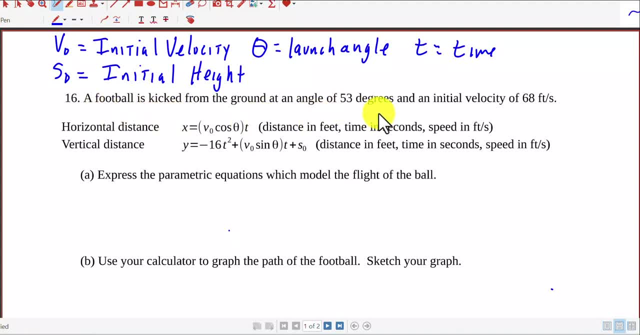 the ground at an angle of 53 degrees and with an initial velocity of 68 feet per second. We'll give you the equations for both the horizontal and the vertical distance. So the horizontal distance, or our x, is v sub 0, cosine theta t, That's our distance in feet, and time is in seconds and speed. 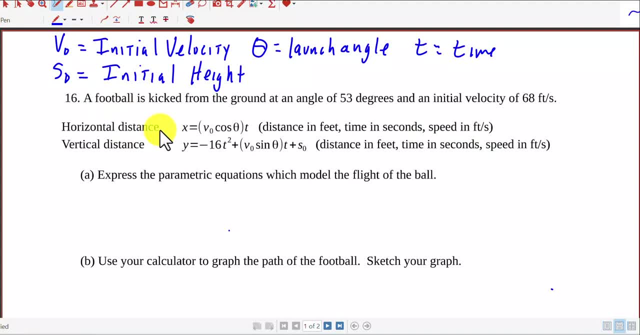 is in feet per seconds. So horizontal distance might be how far something goes, A baseball, how far it is hit, In this case of football, how far it is kicked. And then we have the vertical distance, which is our y, Which is going to be our height, How high the ball goes or how high something is hit. So y equals 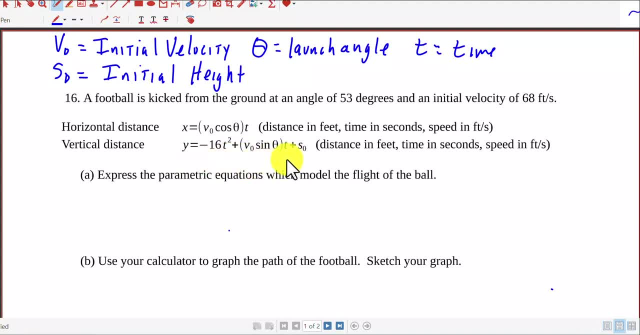 negative: 16 t squared plus v sub 0, sine theta t plus s sub 0.. And again, that's distance in feet. Our time is in seconds and our speed is in feet per second, So we got to have the correct units here. 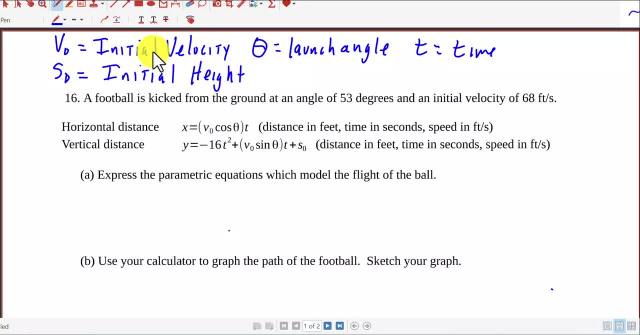 So, just as a matter of identifying things, Our initial velocity is v sub 0.. Our theta is our launch angle, t is time and s sub 0 is our initial velocity. So that's our initial velocity, So that's our initial height. So we want to express the parametric equations which model the flight of. 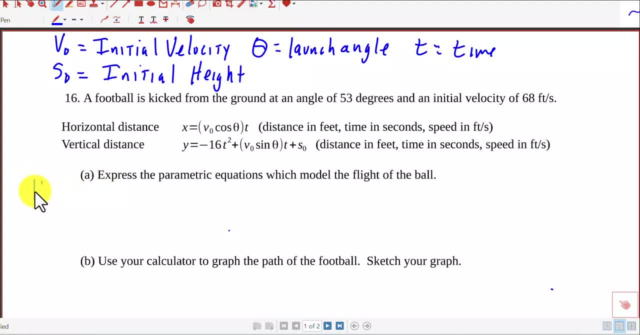 the ball. So our horizontal flight is: x equals 68 cosine of 53 degrees times t, And our vertical distance, Or how high it goes, y, equals negative 16 t squared plus 68 sine of 53.. And that's all times t. 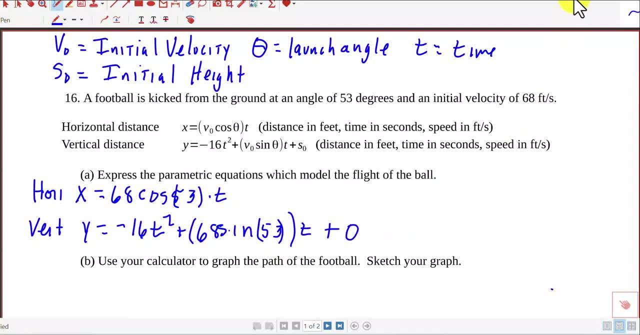 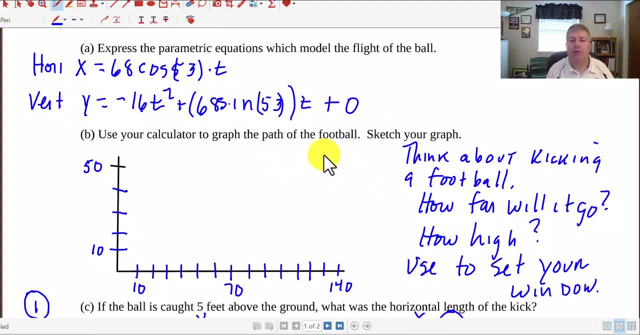 And then plus zero. You don't really need the plus zero. Next, we'll use our calculator to graph the path of the football. So we'll use our calculator to graph the path of the football And then we'll make a sketch of that graph. 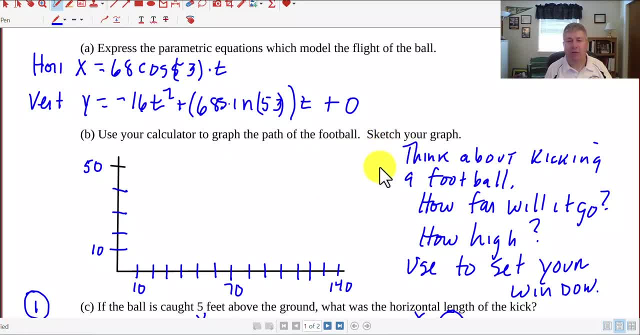 In setting up your window, Think about kicking a football. How far will it go? Well, how far it will go will be what you want to set your x-axis to, Because that's your x values. is that that horizontal distance? And then also think about how high it will go. How high is that gonna go on the 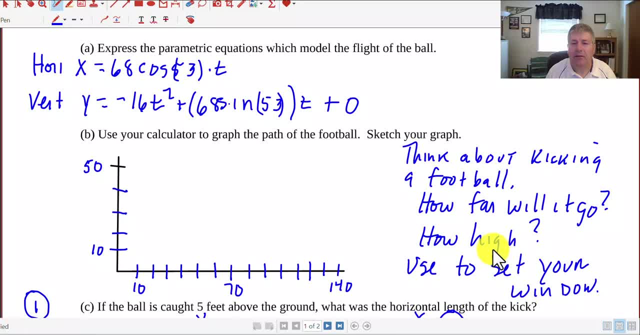 on the y-axis, So use that to think about setting your window. So I did take the liberty of setting some things here on our on our graph. If you kick a football about 50 feet high, that's going to be pretty high, and if you kick it 50, 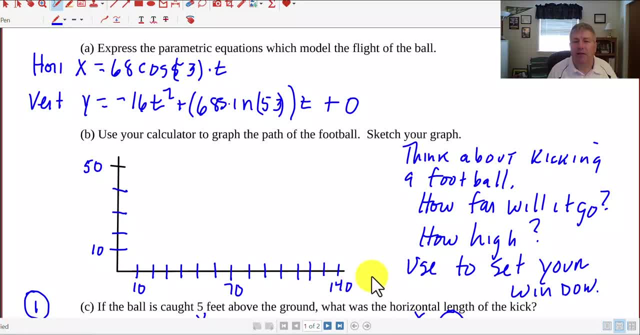 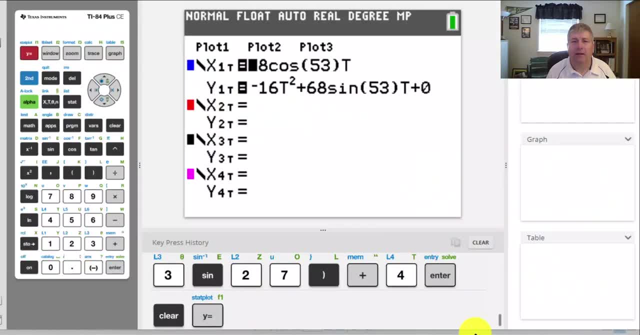 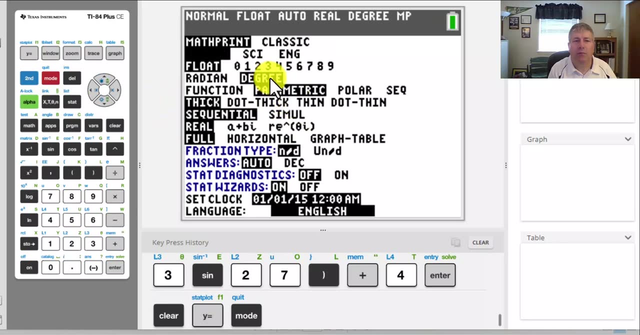 yards, that's going to be about 150 feet. That's a pretty long way. Let's start with with that and we'll head over to our calculator and get things underway. I went ahead and I've set my calculator to the parametric mode and degree mode, so 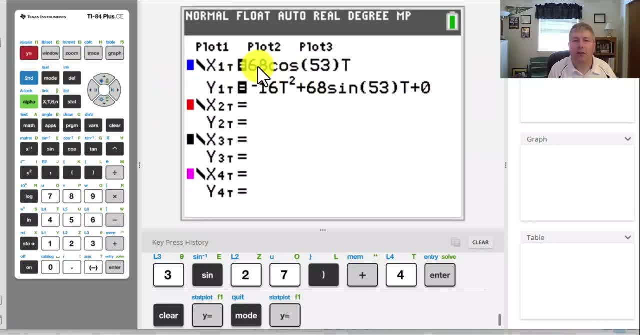 that is done and then I input my two equations. I put my, my x equation for my, my horizontal distance, 68 cosine of 53 t, and then my height, my y, my vertical distance, negative 16 t squared plus 68 sine of 53 t, and then go ahead. take a. 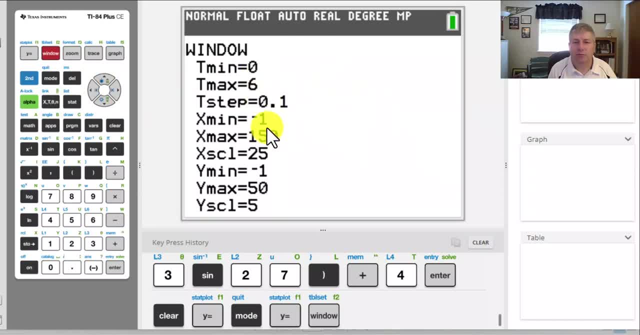 look at our window- went between zero and six seconds. The x min I went, negative one and my x max 150 feet or about 50 yards, And I can change my scale here. since I have it by tens on my graph, I'll change. 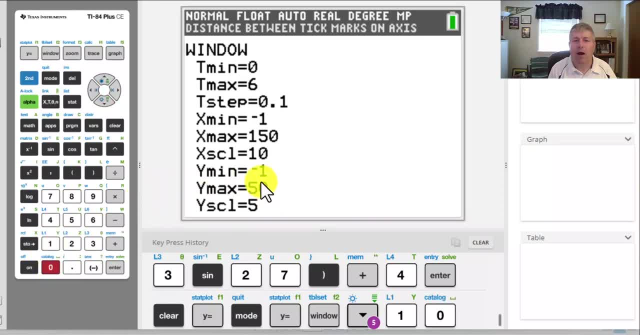 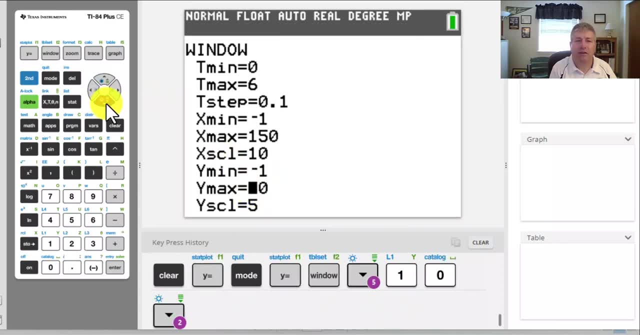 my x scale to 10 and then my y min. I just like to see the y axis and then a maximum height of around 50 feet, and since I had my scale by tens, I will set that by tens and then we can go ahead and graph and see what we see what we. 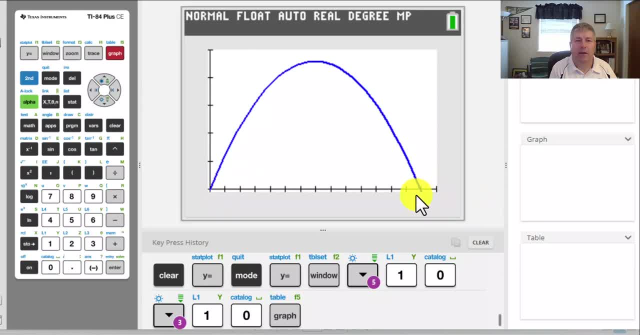 get here, So we get a pretty nice looking graph. it looks like it's gonna go about 40 feet and it looks like it's maximum height will be around between 40 and 50.. We have a pretty good window here, and then you can- you can certainly use the. 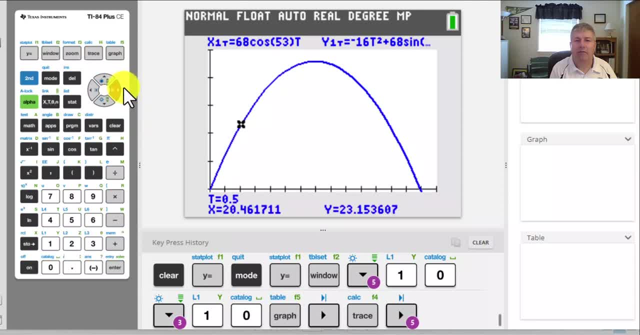 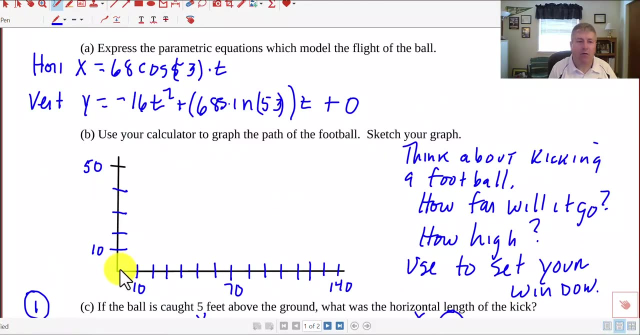 trace key and you can trace along here and find different x and y values at at particular times. We've got some helpful information from our graph. so we go back and we sketch our graph and since we kick it from the ground, the graph is going to look something like this: So we're going to go back and we're going to 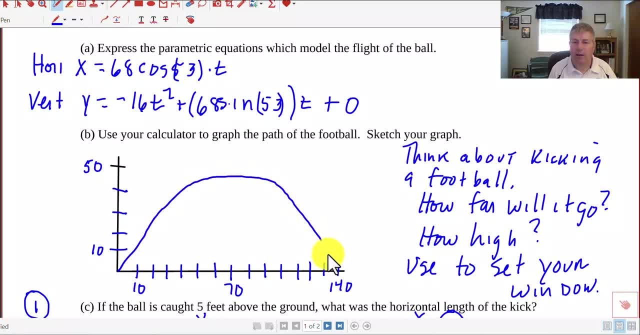 mark it with. what we get is a point on the graph, and then we're going to mark it on the product id. now we're going to take our graphic label and I'm initial on this one. that is something like that, and that's a pretty decent sketch of 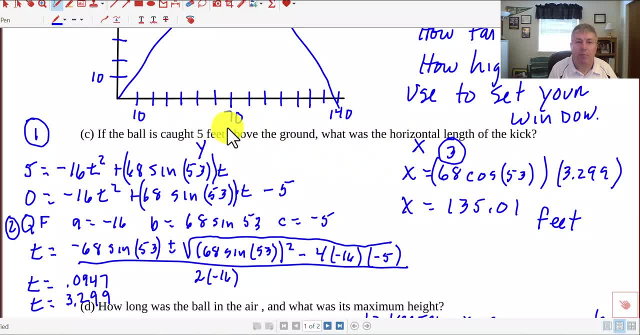 what we have here with our label. so make sure your label and put your tick marks and everything on your graph. now, if the ball is caught five feet above the ground, what is the horizontal length of the kick? Well, five feet above the ground, that five feet is a Y and the horizontal length is an X. So what we need to do here is we need to find out at things like this, 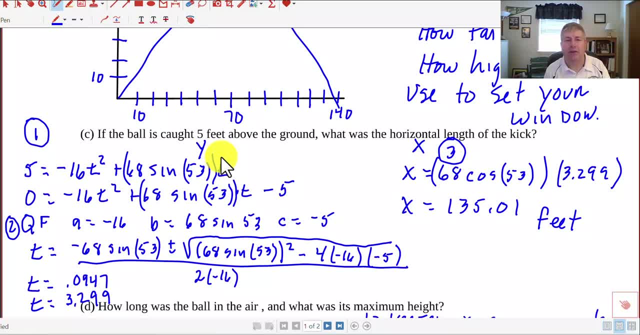 what times the ball is five feet above the ground, because we can see here it's going to be five feet above the ground twice on the way up and then back on the way down. Because five feet above the ground is a y, we'll use our y equations, set it equal to five and solve for t. So I subtract five. 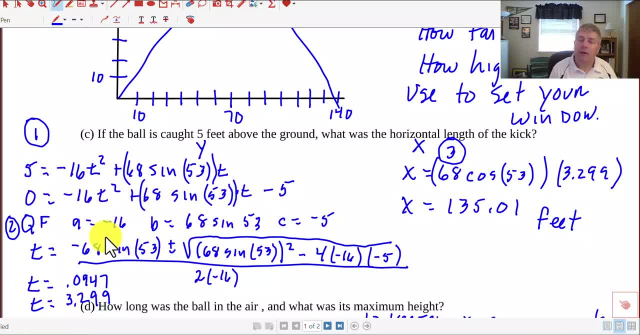 from both sides and I've got a quadratic equation. so we have to use the quadratic formula. So we substitute everything into the quadratic formula. So our a value is negative 16,, our b value is 68 sine of 53, and our c value is negative 5.. So I substitute all that into the quadratic formula. 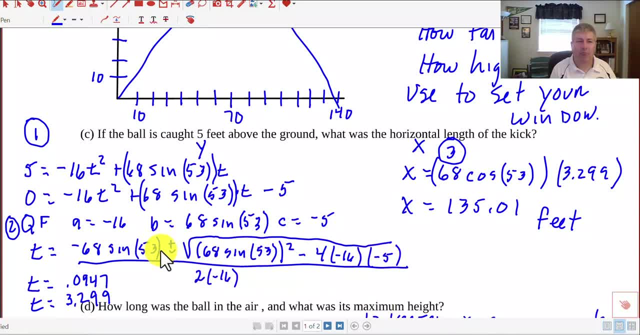 and I did it twice on my calculator, once for the plus and once for the minus, and I get two different times. I got a time of 0.0947 seconds and 3.299 seconds. So write it down and see what happens. So I have a times of 0.0947 seconds and 3.299 seconds. So 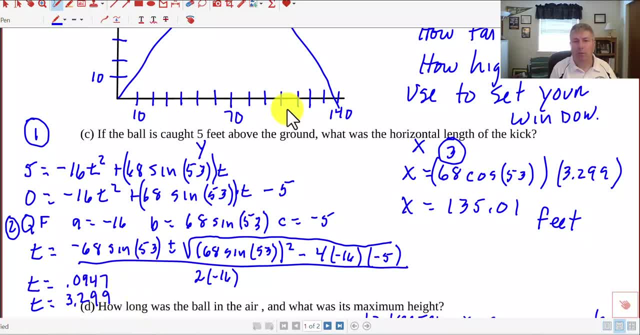 at the beginning, right right after we kick it, and then probably towards the end here when it, when it lands, because it's five feet right before it hits the ground again. so so now I've got my two times, but now I need to find the horizontal length, I need to find the X. so I'm gonna take the second time and 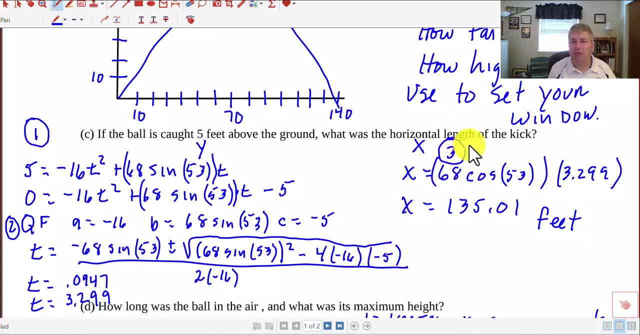 I'm gonna substitute that into my X equation. so that's the third thing I do solve for the X. so X equals 68 cosine of 53 times 3.299. now be sure not to multiply your angle by the 3.299. that's the whole value. so you could even put: 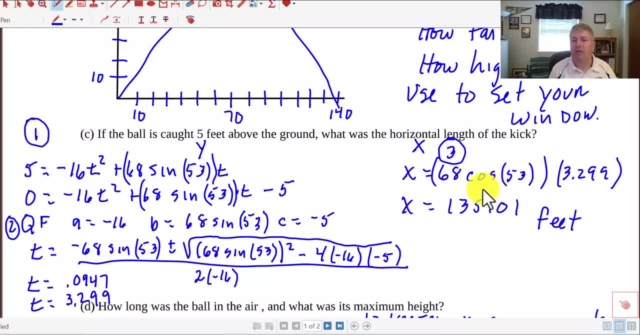 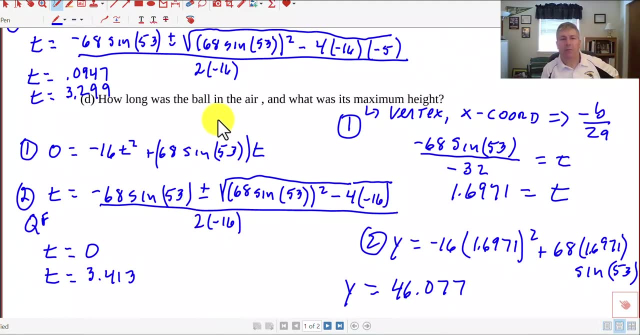 that 3.299 in front, we put that in our calculator and we get X equals 135.01 feet. so a lot of calculator work here and in Part D. D asks how long was the mountain ball in the air and what is its maximum height. so let's answer the: how long the 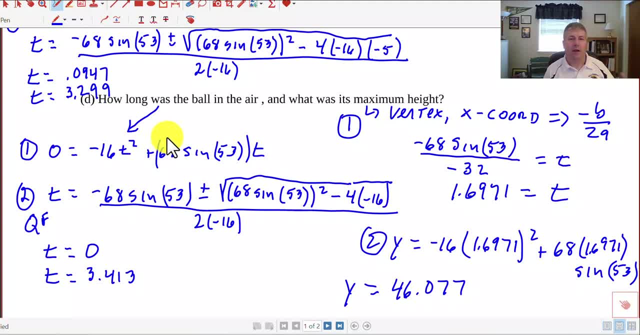 ball was in the air. question first, the. the ball is in the air from when it's kicked until it hits the ground again. so the ground has a height of zero. so we'll use our Y equation for for our height of zero and use that to back into the time. 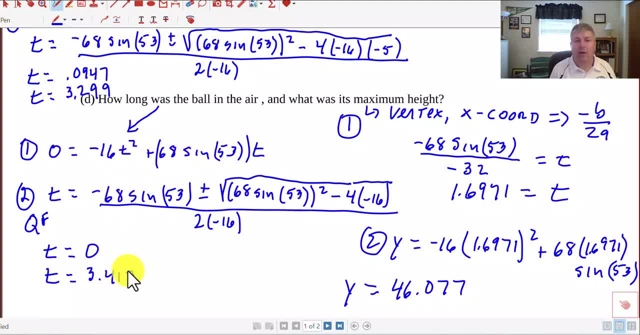 once we know that the the start time and the finish time, well then we know how long the ball is in the air. we should know right off the bat that, well, at times, zero, the height is 0 because we're kicking the ball from the ground, we're. 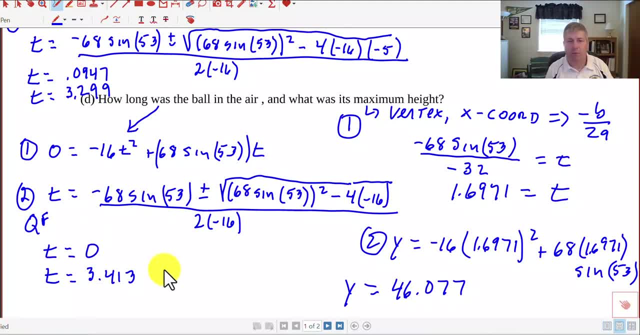 not kicking it from a balcony or above the ground or from the basement level or something like that. we can just substitute everything into our equation. we really are only substituting Y in right now or zero and then substitute into the quadratic formula: our B value is negative, 68 or the. 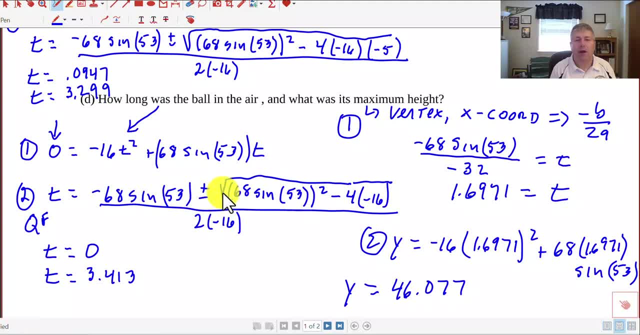 B value is 68, sine of 53, plus or minus the square root of B squared minus 4AC, all over 2A. So be real careful about how you input into your quadratic formula And we get a T of 3.413 seconds. 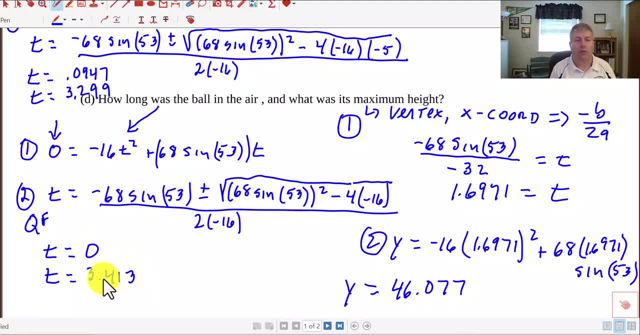 So that's the amount of time that the ball is in the air, between 0 and 3.413.. So the answer to that first question is: 3.413 seconds is the amount of time it's in the air. But now, if we want to find its maximum height, that's going to be a different situation. 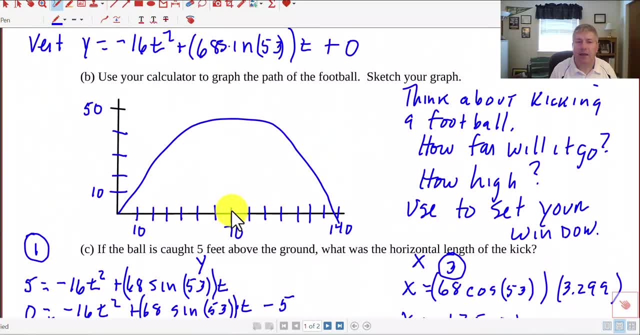 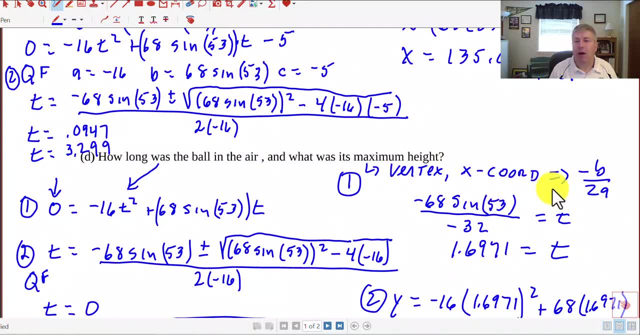 We want to find that peak height, that maximum height. Well, when does that happen? At what time? We can use from our quadratic formula or from our parabola days. the X coordinate of the vertex is the opposite of B over 2A. 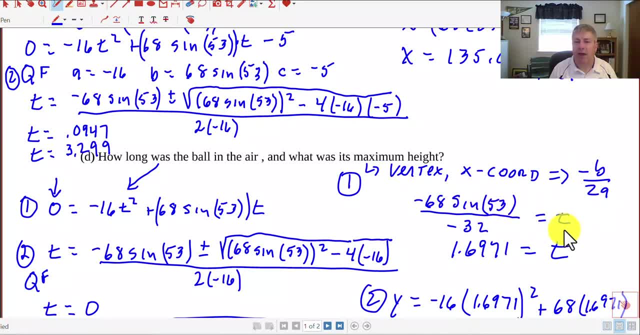 Use the opposite of B over 2A to solve for that value of T. And that's it, And that's it, And that's it, And that T is 1.6971 seconds. I just put in my calculator negative 68,, sine of 53, all over 32,. 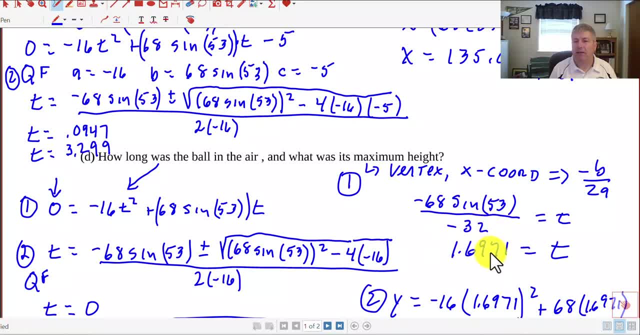 because our B value and then 2A. So we calculate that T. Well, now we want to find the maximum height. Well, height is a Y, But I've got the T, So a little bit different. We're going to use the same formula but we're going to substitute in for T.